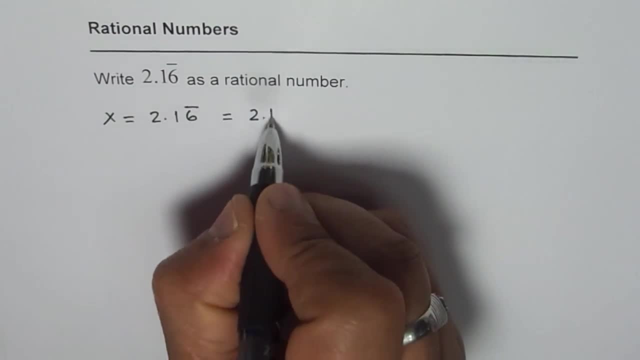 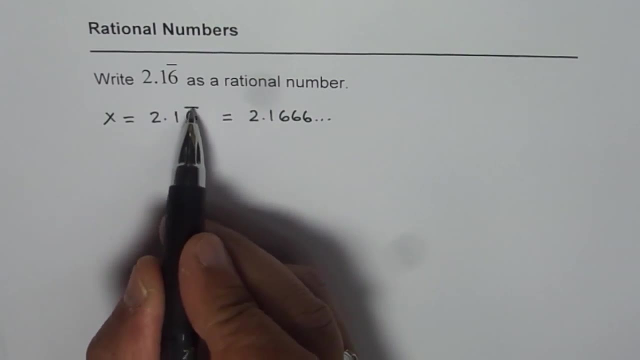 It really means the number is 2.1666, like this, correct? That is the meaning of recurring This bar on top of 6 refers to repeating 6.. Now the strategy is we should actually multiply this by 100 so that we get 2.16 and 6 recurring after decimal. So we have 100 x equals to 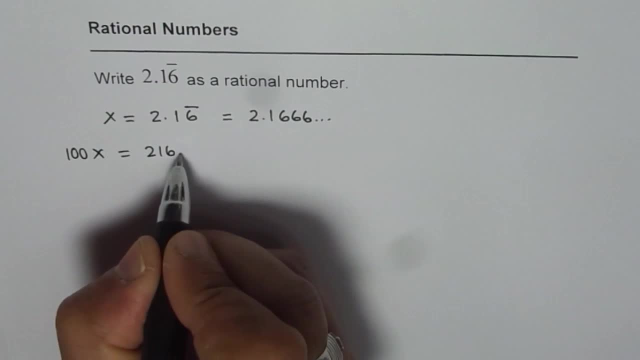 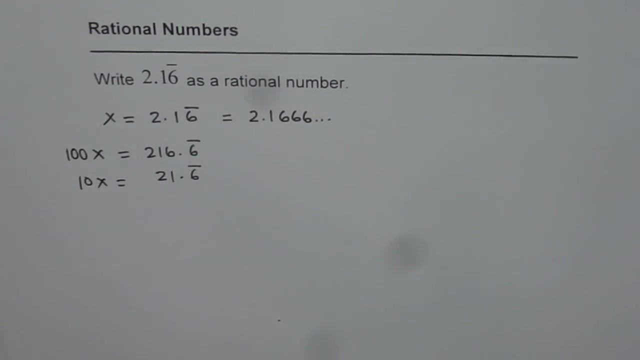 so it becomes 2.16.. 2.16 to 116.6 recurring. We can also multiply this by 10.. If I multiply this by 10, I get 21.6 recurring. Now what is 100 x minus 10 x? That is to say, we'll take away 10 x from 100 x, Then we 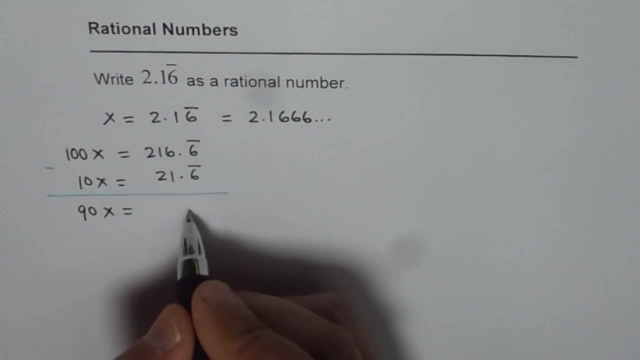 get 90, x equals to anything after decimal is 6 recurring. When you take away it becomes 0.. And on the left side we get 6 minus 1 as 5, and then here we have 11 minus 2 as 9.. 195. 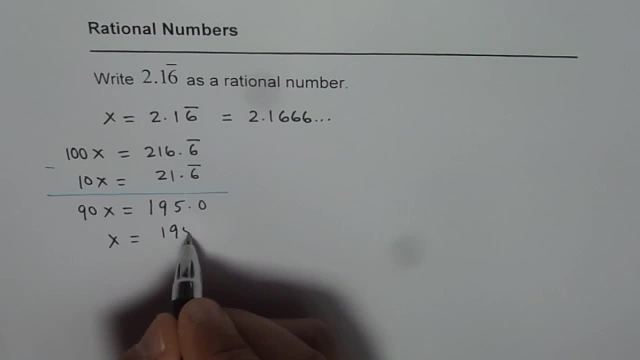 So we can write this as: x equals to 195 divided by 90.. Now it can be simplified: You can divide both by 5.. If I divide by 5, I get 5 times 3 as 15, and then 45 will go 9 times. And dividing this by 5, 5 times 1, and 40 is 8.. So I get 18.. I can further. 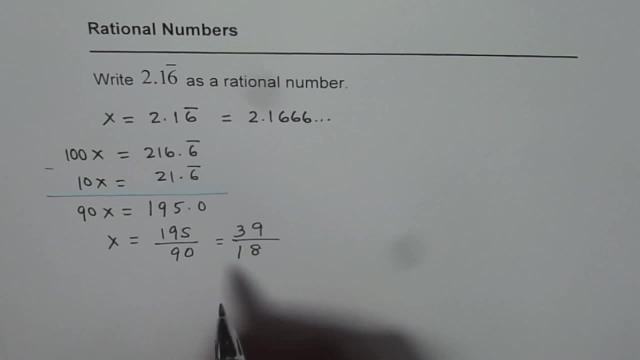 divide this by 3, right, So it gives us 13 here and 3 gives me 9.. So I can write this as 13 over 9.. So sorry, 13 over 6, yeah, So we are dividing by 3, right, So 18 divided. 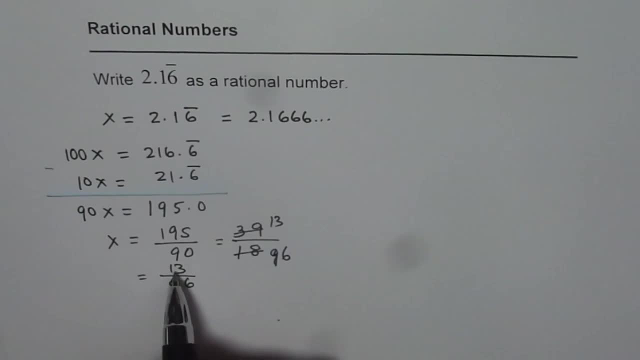 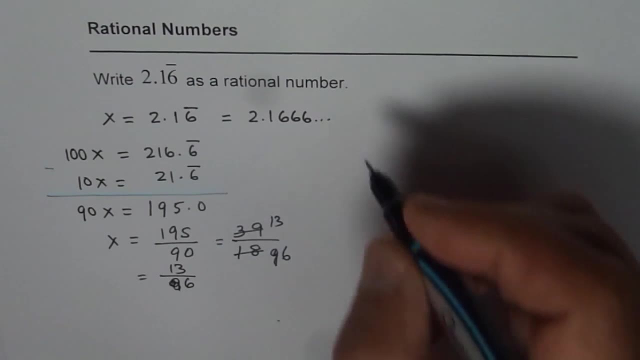 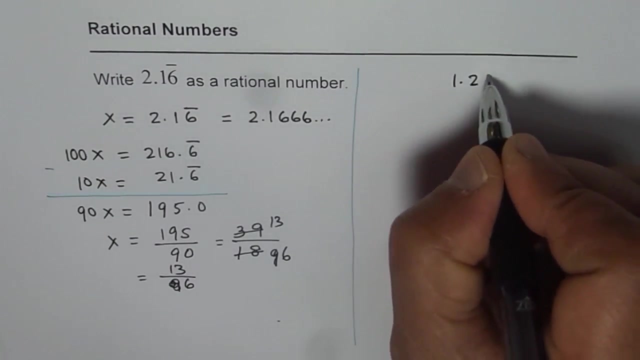 by 3 is 6.. That is correct. That gives me approximately 2 point something right. Twice 6 is 12, and numerator is 13.. That is correct. Let me take one more example and show you again The whole process. This time let's write a number like 1.25, recurring. So let us say: